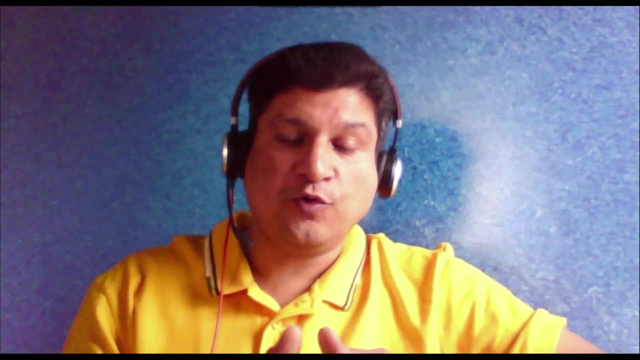 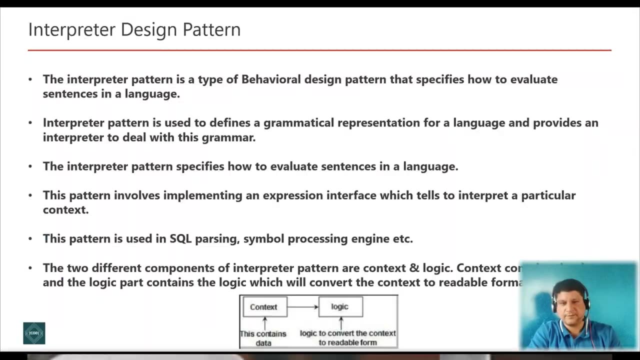 like, share and subscribe my channel so that I can grow Code One Digest family. Thank you, Okay, so let's start with the interpreter design pattern. What is interpreter design pattern? Interpreter design pattern is one of the behavioral design pattern. Interpreter pattern is used to define a grammatical representation for: 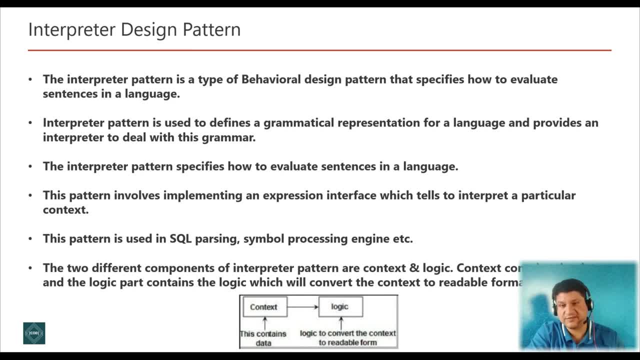 a language and provide an interpreter to deal with this grammar. The interpreter pattern specifies how to evaluate sentences in a language. This pattern involves implementing an expression interface which tells to interpret a particular context. This pattern is used in SQL parsing, symbol processing engine, etc. An interpreter pattern says that to define 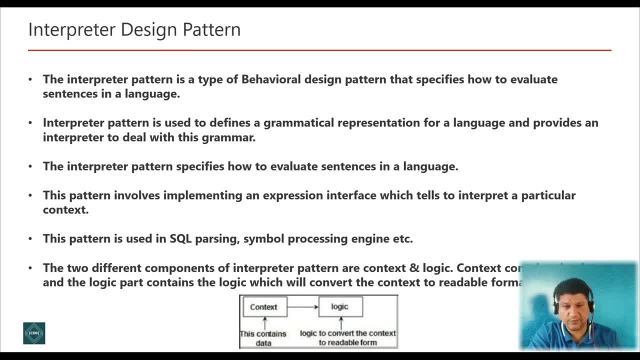 a representation of a grammar of a given language, along with an interpreter that uses this representation to interpret the sentence in language. Grammar are mapped to the classes to arrive to a solution. For instance, 7-2 can be mapped to a class minus. 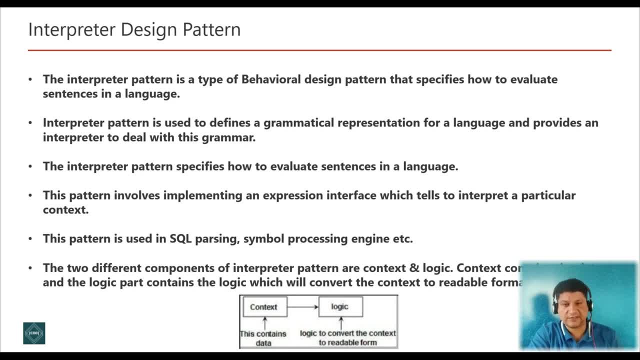 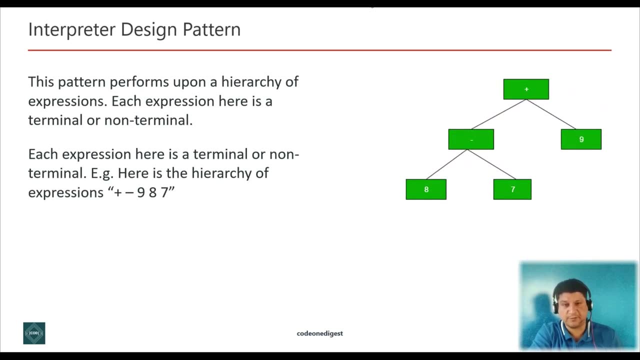 The two different component of interpreter patterns are context and logic. Context contains the data and logic part contains the logic which will convert the context to a readable format. This pattern performs operation upon a hierarchy of expressions. Each expression here is a terminal or a non-terminal component. 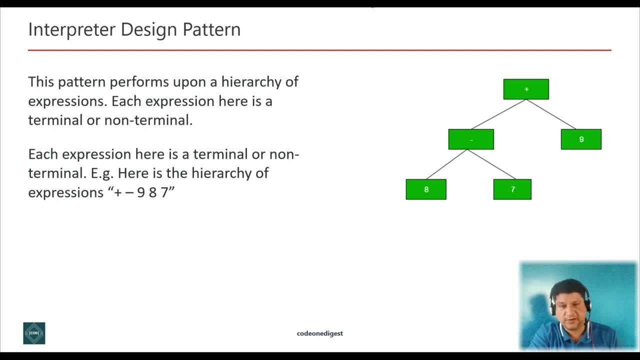 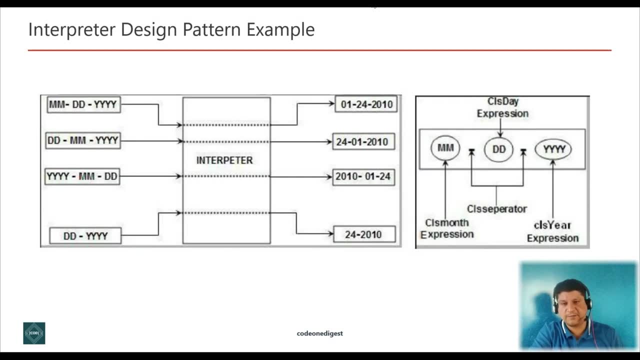 Here is the hierarchy of expression: plus minus 987.. You can see on your screen how it is structured in a tree. Now let's understand interpreter pattern with an example. The example, what you see on your screen. we have broken a date format into four components. 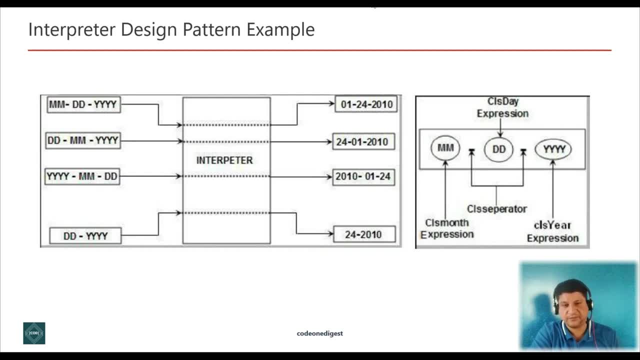 Month day, year and a separator. For all these four components, we will define separate classes which will contain the logic. There are two types of classes. One is expression classes, which contains the logic, and other is the context classes, which contains the data. 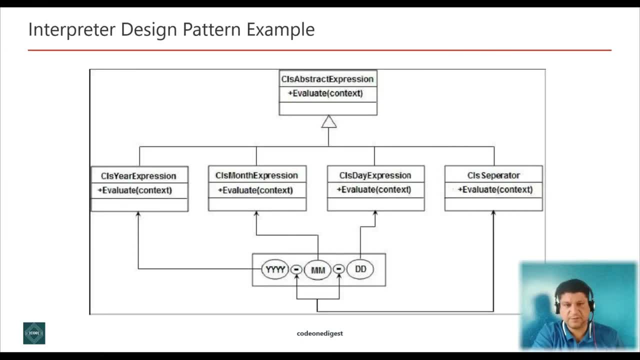 So what we have done is we have defined all the expression parsing in a different classes. All these classes inherit from a common interface, that is, class abstract expression with a method. evaluate. The evaluate method takes a class Once a class is a context class which has the data. this method parses data according to the 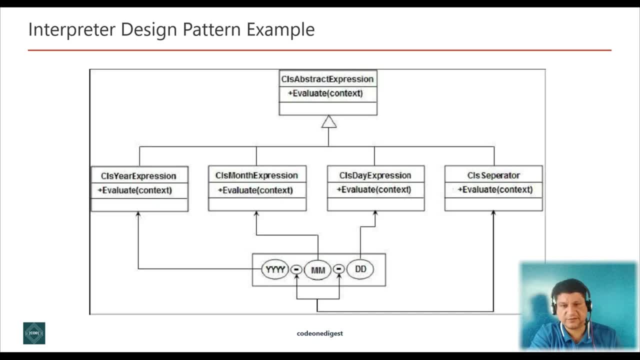 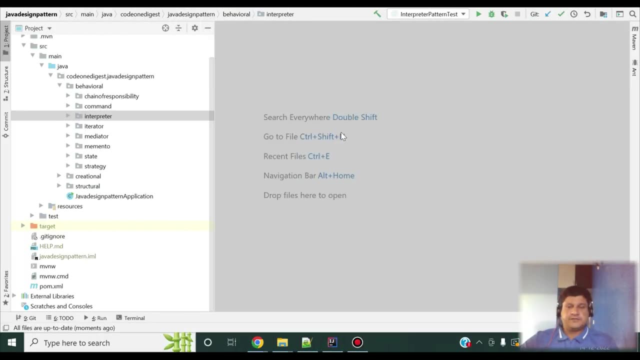 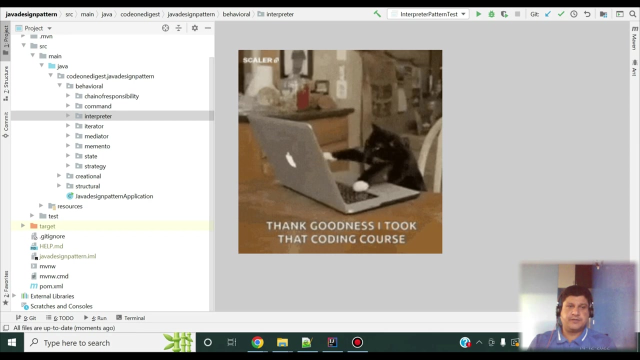 expression logic, For example. Okay, friends, now let me show you the code of interpreter design pattern. What i have done is i have prepared a code for you- you: interpreter design pattern. i'll walk you through this code first and then i'll run and. 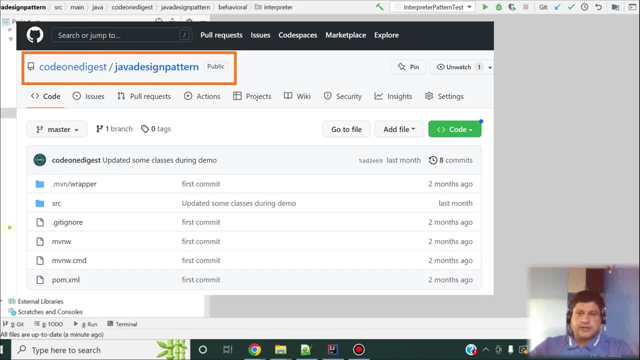 give you the demo. friends. i have shared this code in my github repository. you can download this code and play with it. the link of my github repository is shown on your screen. just use that link to download the code. and also the link is available in the description section. 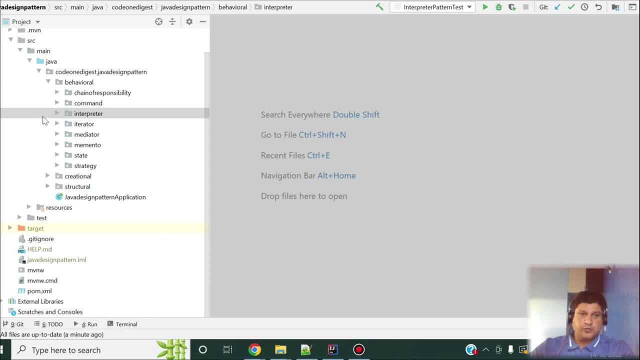 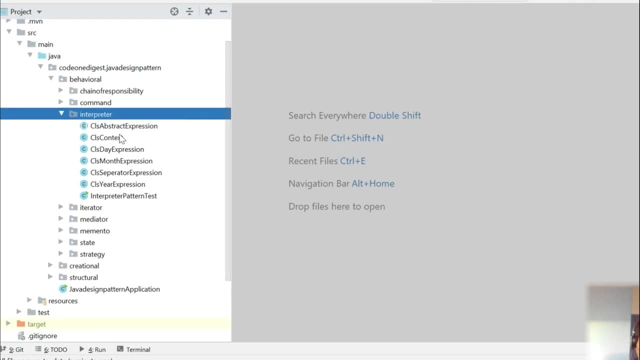 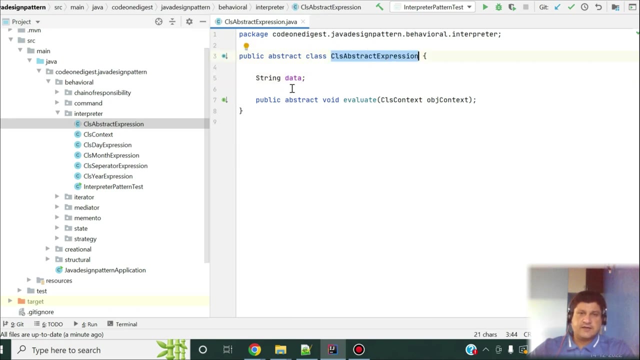 of this video. let me show you what i have done. i have interpreter package where i have all the classes of this demo. i have defined one extra class. we call it class abstract expression. in this class i have one string type of data and i'm having a method evaluate. 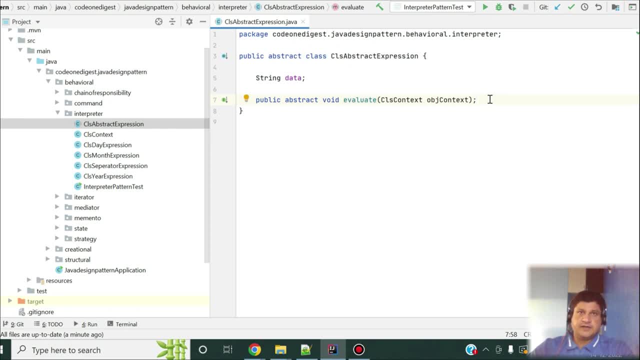 so i'm taking an example of our date. that means date, month and year, and using a date different expression, how can we display the same date in a different, different format? it's very simple implementation of our date format in java, this abstract class and i have three implementation. 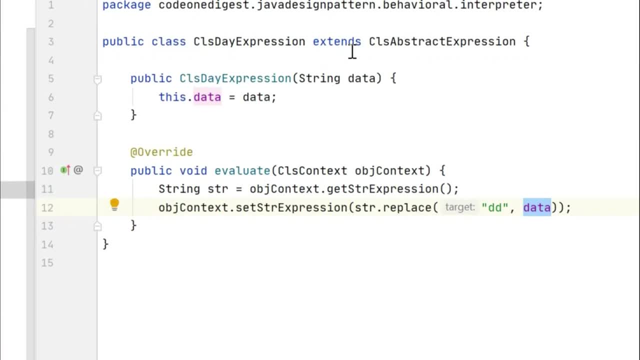 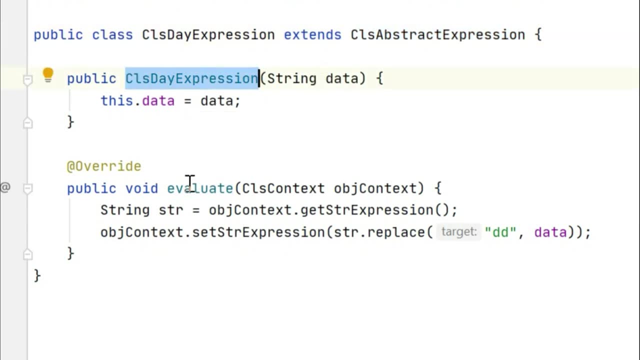 of it. so one is day class, day expression. it is extending that abstract expression where in a constructor i'm initializing the data and i'm overriding, i'm implementing that evaluate method where i'm i'm passing a context. here, context is nothing but my data, my object, i'm retrieving an. 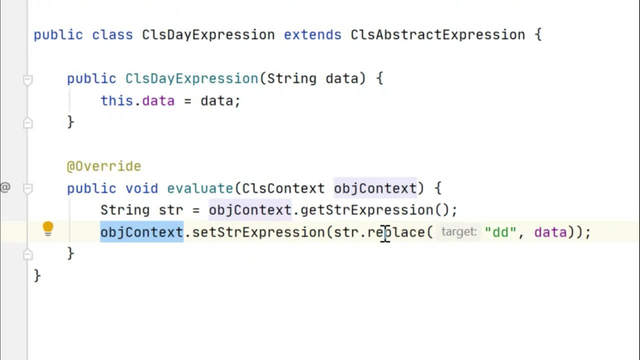 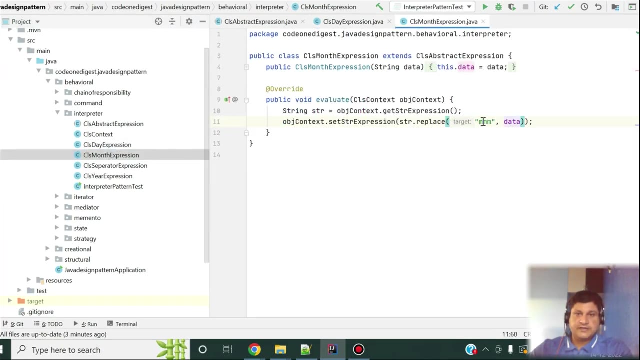 expression from it. and here, at this point, i am replacing the dd with data and setting that in my expression of this context. same thing i'm doing for month, but here i am replacing mmm in the data. okay, and same thing. i'm doing it for year, replacing it with data. now let's see what is. 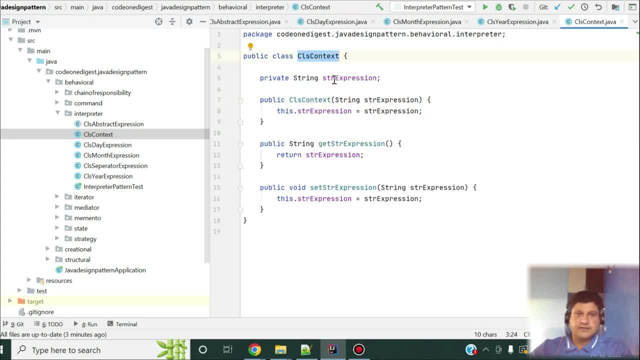 in context object. so in context i'm having one string, string expression. string expression is nothing but in a format in which format we want to see a data. so this context will have that information: that in which particular format i want to see a data. i have a constructor and i. 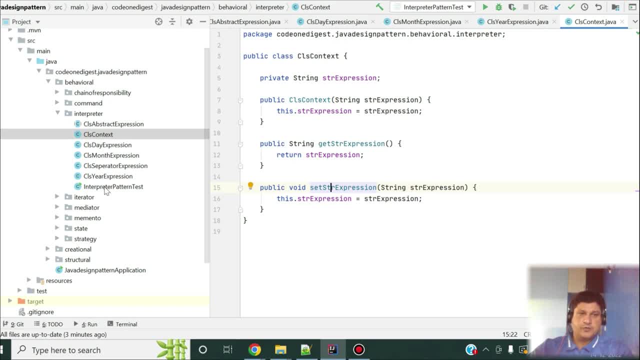 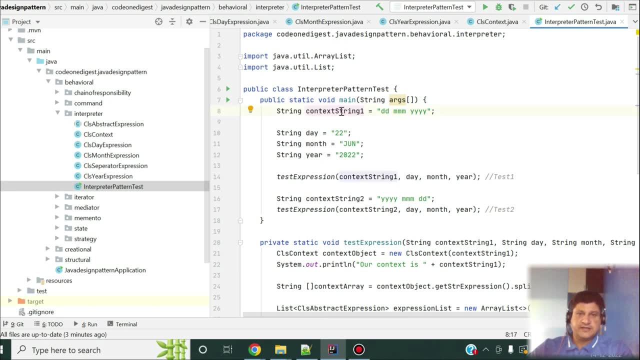 have a getter set of that expression. now i have written a test class. let's see what we are doing in test class. so in test class, i'm defining our expression. this is our first expression, that is ddmm yyy. i want to see my date in this format and this is my actual data: day is 22, month is june and year is 2022. 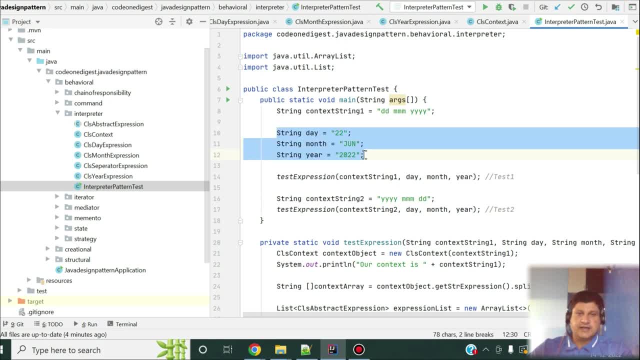 now, using this data and using this expression, i can format this data and i can format this data and i can format this data and i can format this data, this particular date, into this format. this first expression. i also have defined a second expression where i'll reformat the same date into this format. we will see both of that. so this is my. 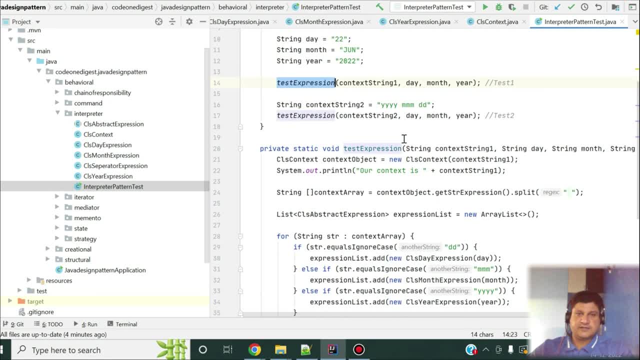 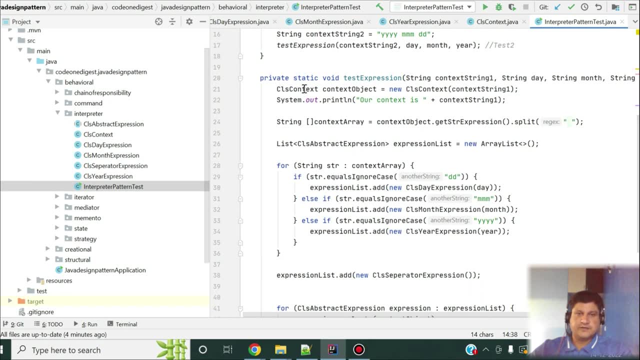 first expression, this is my data and i am calling this method. this is the local method where i'm passing this expression and date, month, year. now, in this method, what i'm doing is i'm creating an instance of my context, i'm passing that my expression here so that it knows, key how i have to format my data. now i'm i'm splitting that. 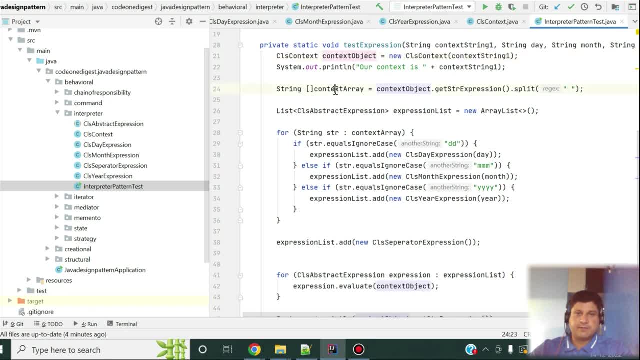 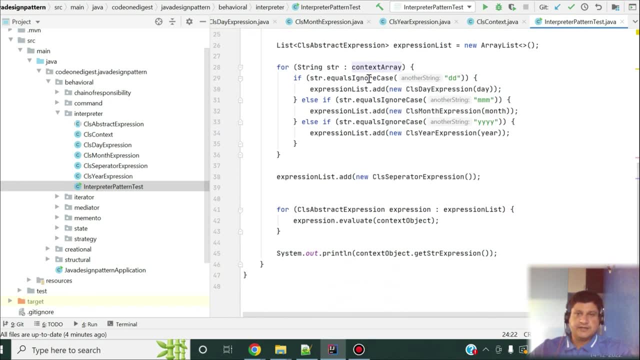 expression with the space, so that i have ddmm, yyy separate in three different component in this array and then i'm iterating it here. i'm checking if a string has dd, then create one instance of a expression by passing the day and day is nothing but our day. 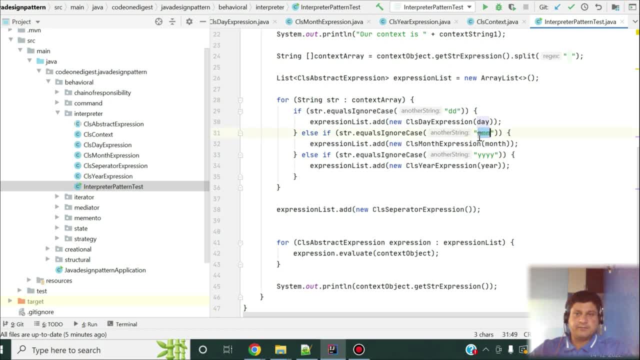 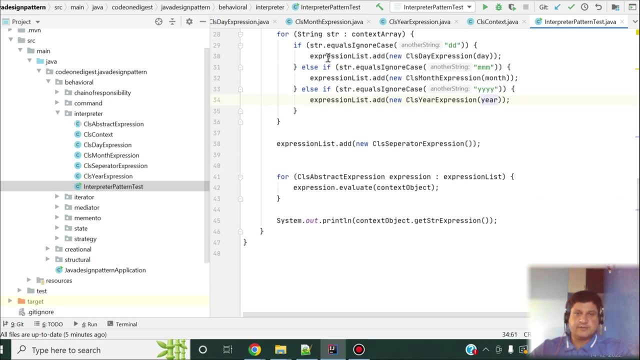 then i'm creating a string and i'm passing the day, and day is nothing but our day. then if it is mm, then i'm creating an instance of month. if it is yyy, then i'm creating an instance of year and passing the year. once this is done, when this loop is executed, i'll call. 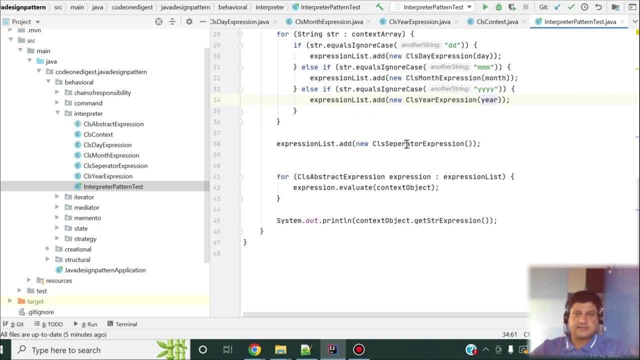 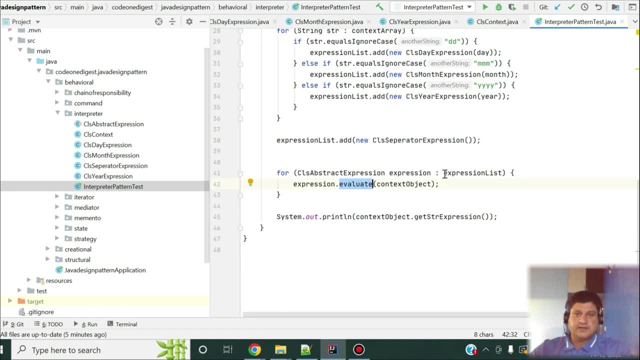 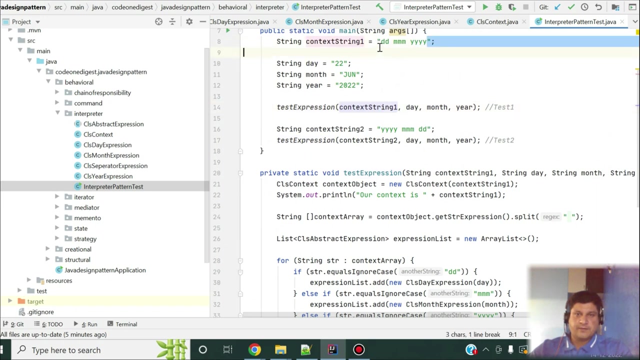 expression list dot. add new cls separator expression, because here our separator is space. now i'm looping this list and evaluating, calling the evaluate method of all, and then finally i'm printing how my date is got formatted. so i'm doing this first for my expression first, and then here i'm doing it. 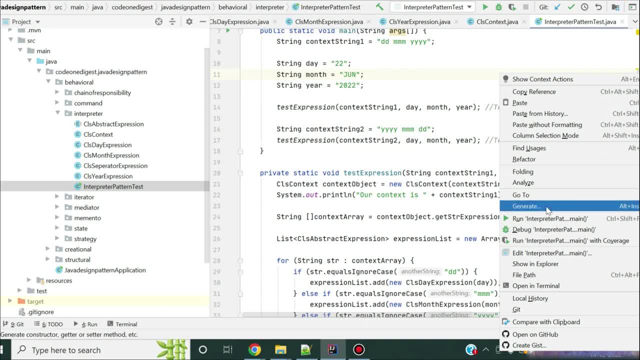 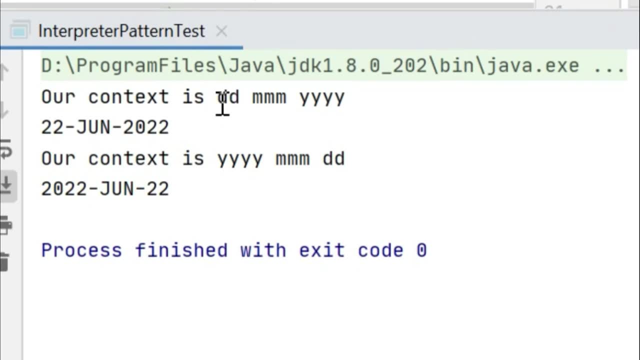 for expression two, let me run this and show you how that works. so do you see that our context expression is ddmm. yyy and whatever data we are giving as a input, it got formatted into this expression: 22nd june 2022. then our second expression was yyymm. dd, so our date got formatted into 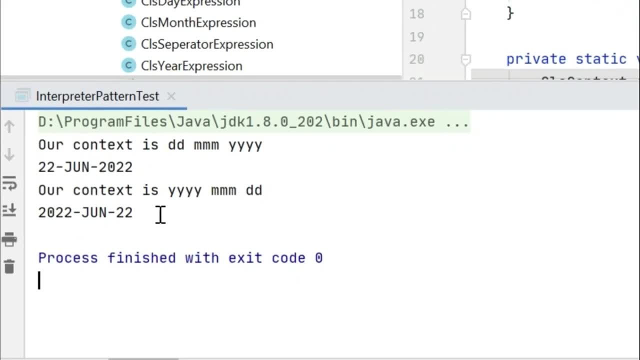 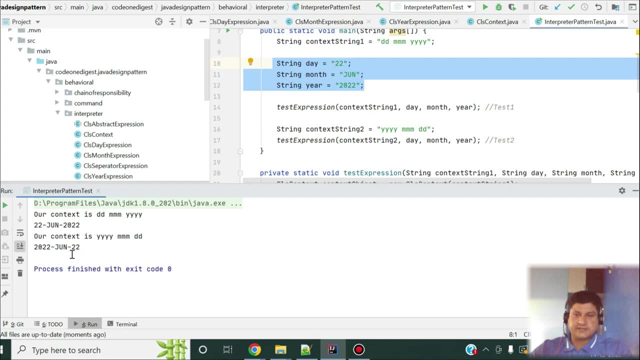 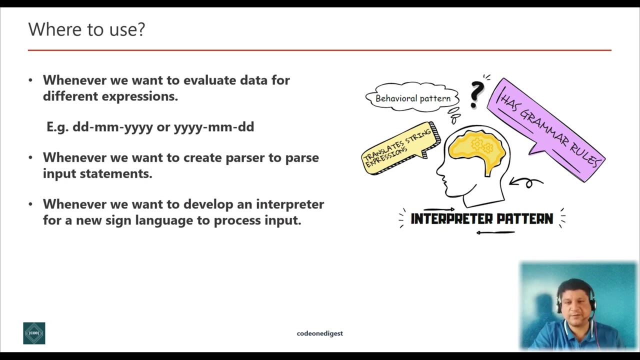 2022, june 2022, like this, right easy. so you may have a scenario where you want to create a parser. there you can use this pattern. so, friends, you may ask where to use interpreter pattern. what is it? the use case of interpreter pattern? so you can use interpreter pattern whenever you want to. 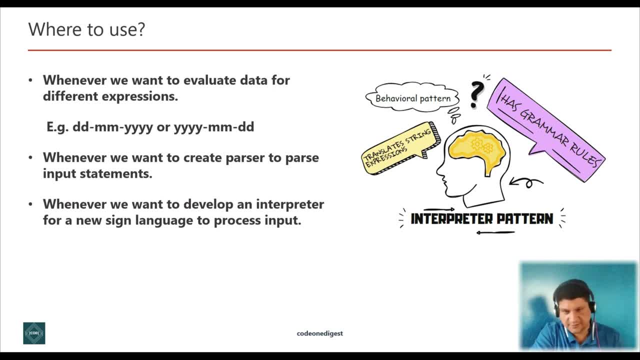 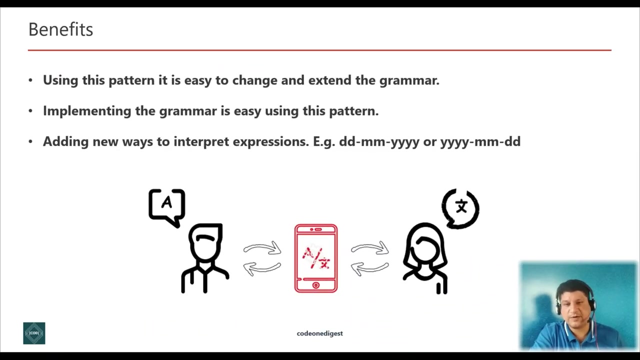 evaluate data for different expressions. whenever you want to create parser to parse statements to take inputs, that time you can use interpreter pattern. whenever you want to develop an interpreter for new sign language to process user provided inputs, that time you can use interpreter pattern. so what are the advantages we get from interpreter pattern? it is easy to change and 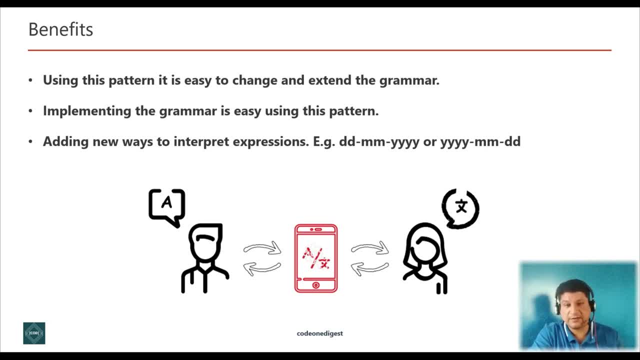 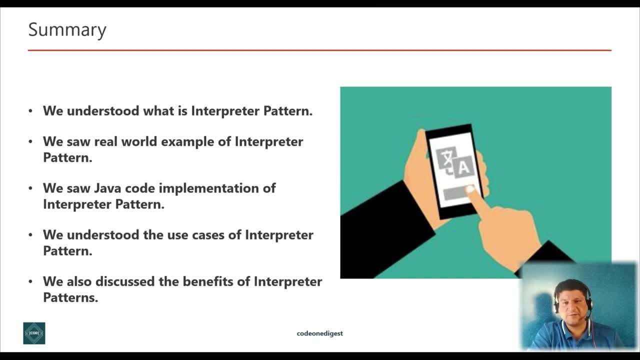 extend the grammar. it is easy to implement the grammar and is easy to add a new way to interpret expressions. friends, now let me summarize what we learned in this video. we understood what is interpreter pattern. we saw a real example of interpreter pattern. we also saw java code. 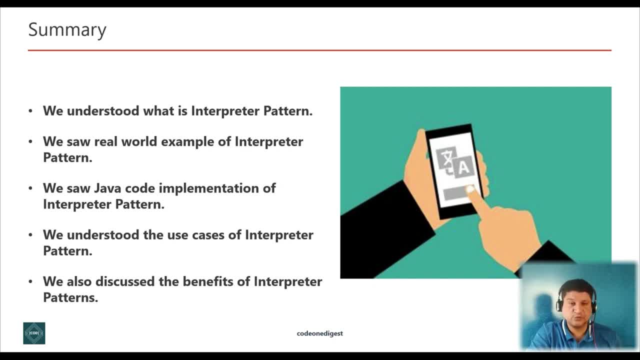 implementation of interpreter pattern and we saw the use case of interpreter pattern and at the end we discussed the benefits of interpreter pattern. friends, let me know if you have already used this pattern in your project or come across a scenario where this pattern can be useful. please reply in the comment section with your answer. 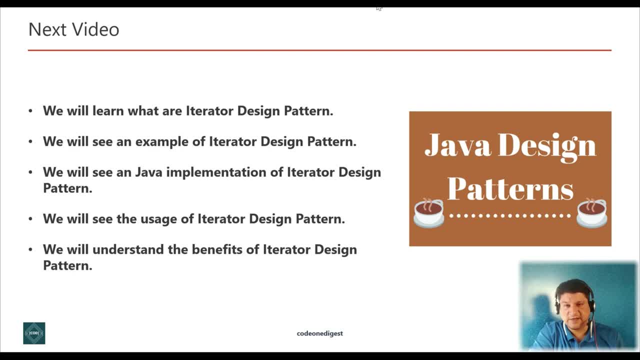 in the next video we will cover iterator design pattern. so we will learn what is iterator design pattern, we will see the usage of iterator design pattern. we will also see a java code implementation of iterator design pattern and we will understand the benefits of iterator design pattern. so stay tuned for the next video and do subscribe to the